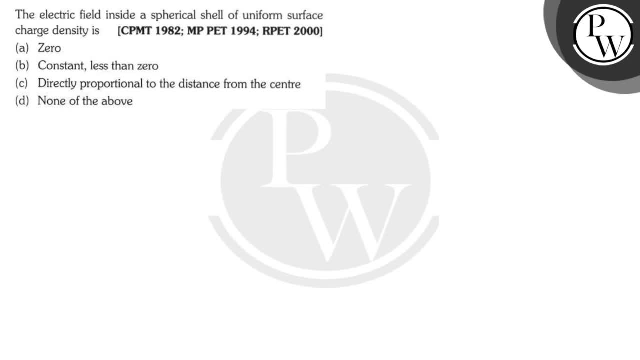 Hello bacho. let's read this question. The electric field inside a spherical shell of uniform surface charge density is given by which of these values? So in this question we can draw the diagram. We have a sphere which has some positive values spread across. 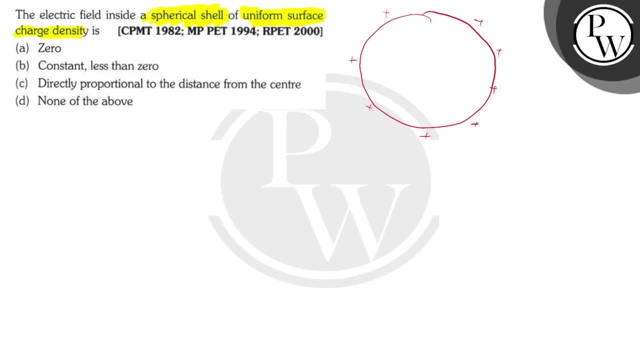 So we have: this is spread across uniformly, and this is the center. So we have an imaginary shell inside this, at which point we have some field E. Right, this E is constant at any point of this imaginary circle because this charges uniform. So since this charge is uniform, we can say that the electric field will be. 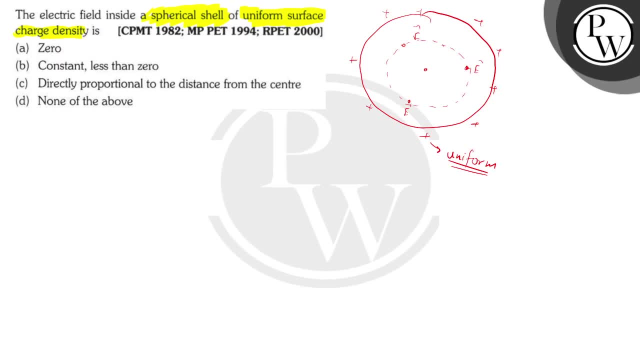 symmetrical across this imaginary spherical shell. Let the radius be A, So using Gauss law, we can say that E dot dA, the integral, which is the flux, is going to be equal to Q enclosed by epsilon naught. So Now we have this E dot dA, Since E is constant throughout this whole imaginary spherical shell. 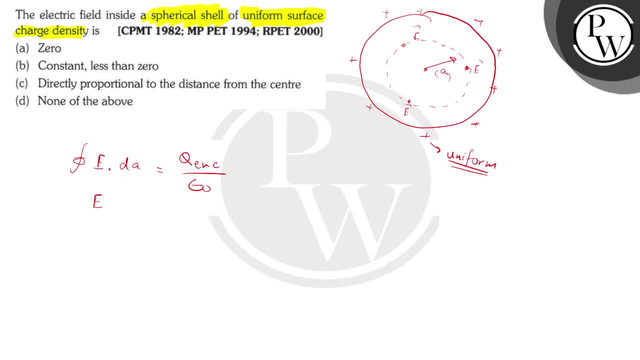 we can take it out of the integral and then we will have integral of dA. Integral of dA is nothing but the area of the imaginary spherical shell which will become 4 pi A square. This is nothing but equal to Q, enclosed, divided by epsilon naught. Now, as you can see, the charge is completely. 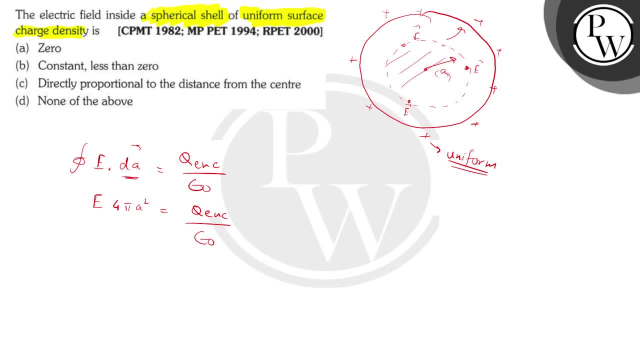 outside the spherical shell. So inside the Q is equal to the Q. enclosed is equal to 0.. So we can say the right hand side is equal to 0.. Now on the left hand side we can say that 4, pi and A square, these are all finite values. These are all finite values, So that means E has to be. 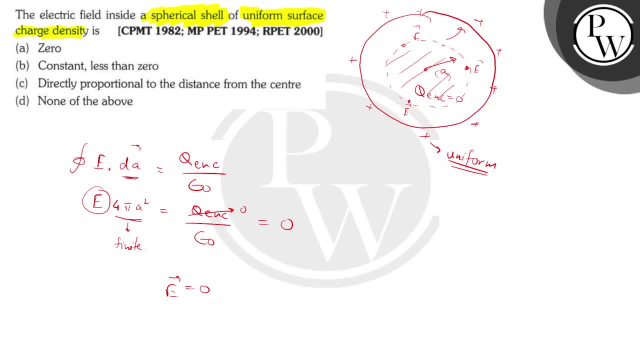 equal to 0. So we have got: E is equal to 0.. So for any radius A, we can say which is still infinite. So we can say that E is equal to 0.. So for any radius A, we can say which is still.